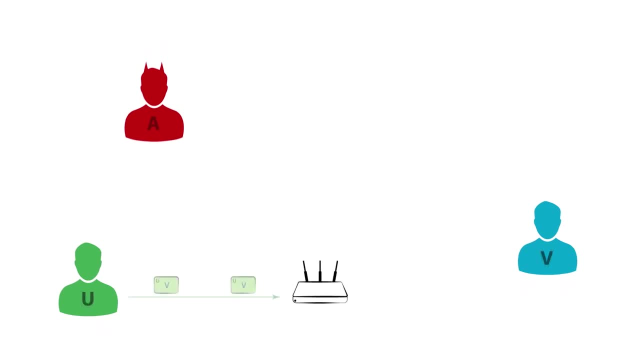 it in a mailbox. Now, if someone wants to disrupt or completely disconnect someone else's Internet service, they can send packets with a fake source address to that victim- So many packets that the victim has no resources left to process legitimate packets. An attacker can even use many different fake source addresses across. 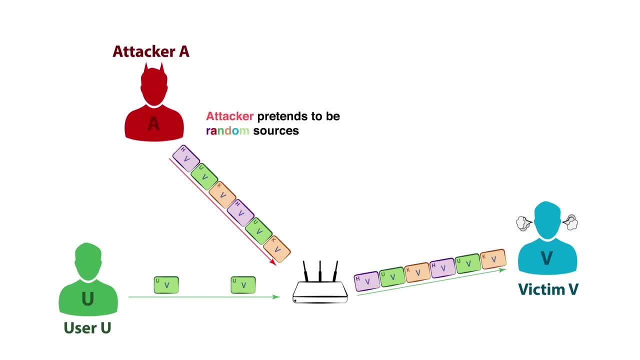 many packets, making it operationally infeasible to trace back the attack to its origin or to block the attack at the victim. It gets even worse. An attacker can commandeer intermediate nodes to amplify an attack by triggering that node to send the victim back. 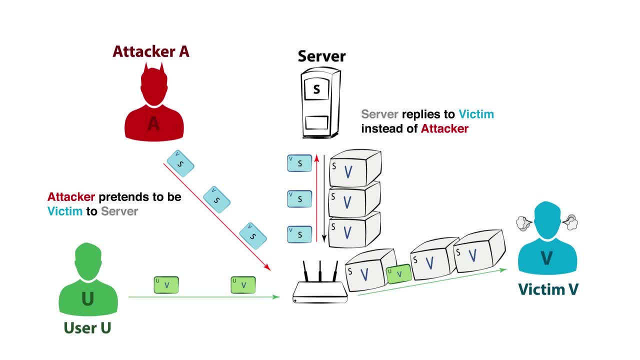 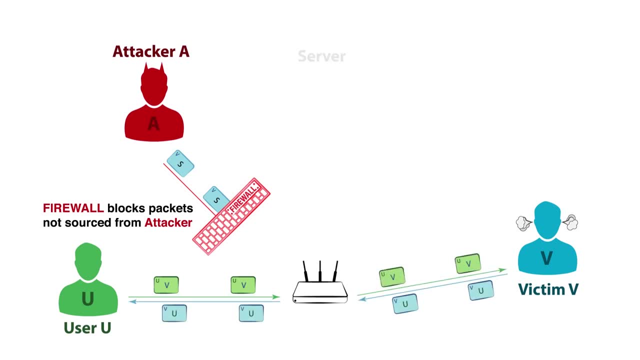 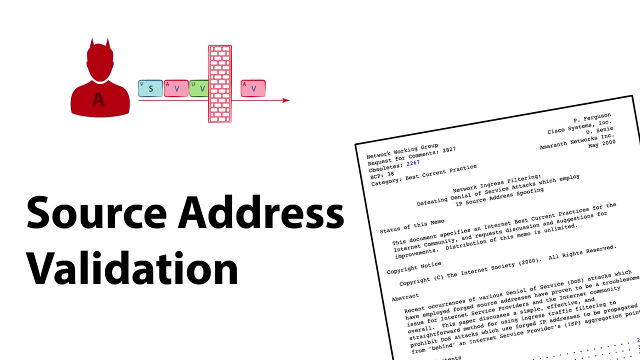 to the victim. The only way to block such attacks is at or near the source, every source, because only those networks near the edge know which addresses are legitimately supposed to be source addresses in packets leading those edge networks. Unfortunately, such blocking or source address validation, although a well-known best practice for decades, is an example of 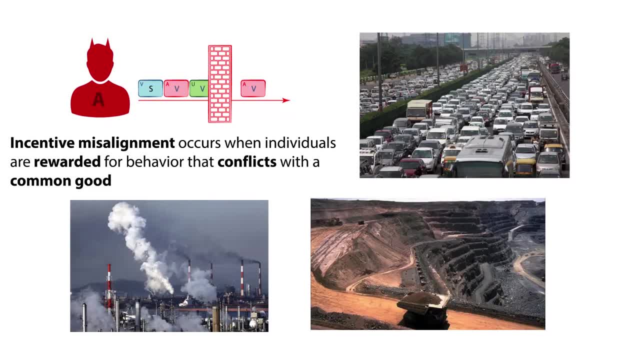 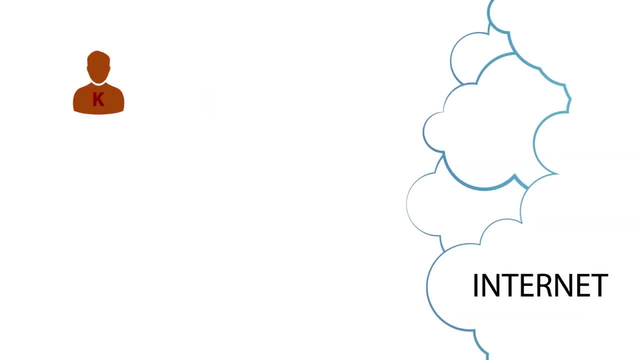 classic incentive misalignment, Because deploying source address validation is primarily for the benefit of networks other than the one deploying it. And, although many networks do filtering, there is no way to comprehensively measure the extent of deployment of source address validation without crowdsourcing volunteers to download a tool that attempts to send a packet with a fake source address. 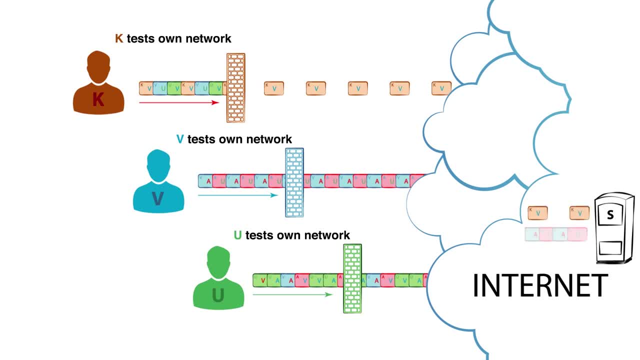 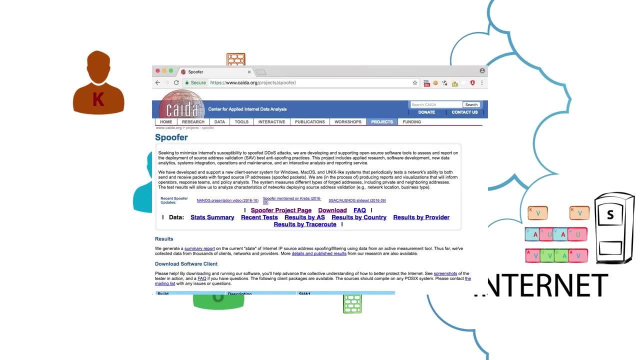 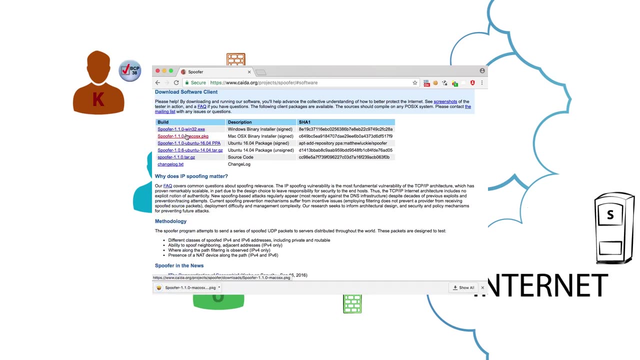 to a known server and then analyze which packets make it to the server. That is essentially what KEDA's spoofer measurement system aims to do. To implement the spoofer system, we have developed end-user tools and supporting back-end infrastructure to allow us to crowdsource the measurement of source address validation. 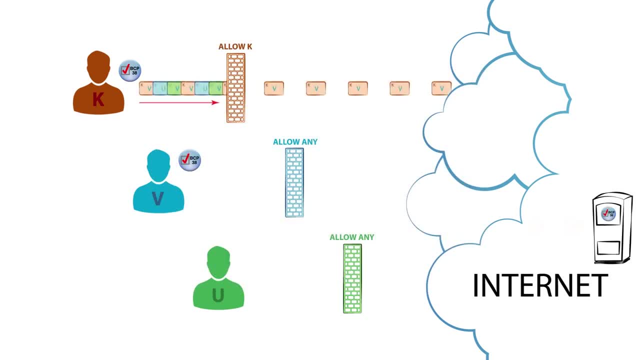 deployment across the internet. We analyze the results of these measurements to target remediation efforts where they can have the most impact. Many networks are using our tool to help fix their own network configuration and make sure source address validation is working, And many other networks have no idea that they have not configured source address. 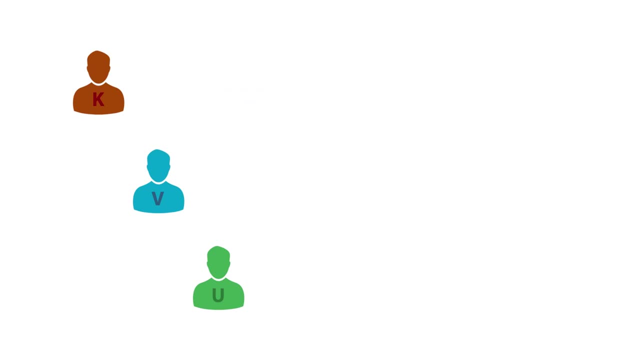 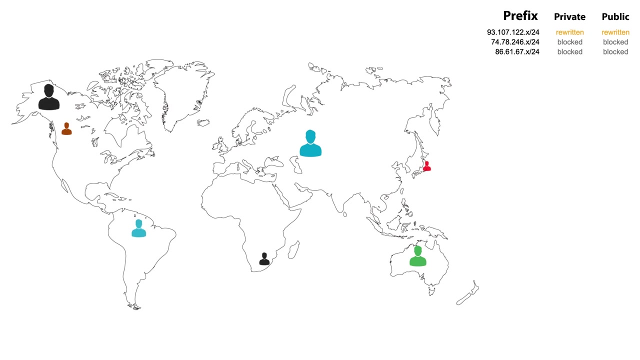 validation correctly. The most important thing we need now is many people to run our tool, which should take you less than 60 seconds to install. Once installed, it will run in the background testing any new networks you visit. We have only recently started and are already gathering.